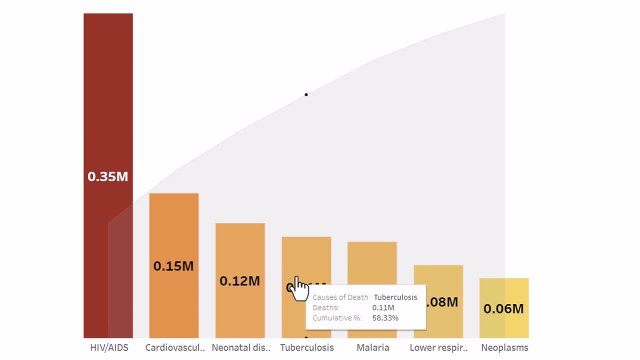 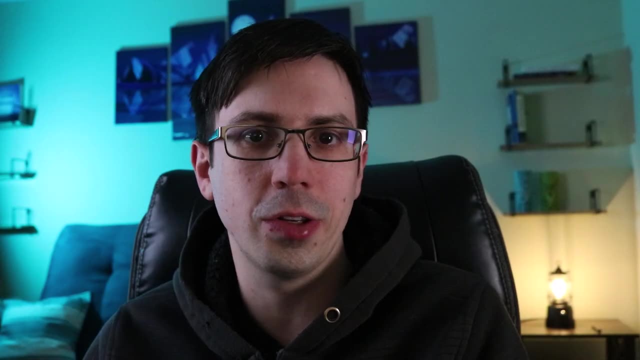 countries tend to be from things like HIV or malaria. This is an eye-opening data set that really lends itself well to the data set and I'm going to talk about it today. So let's get started. I actually have a video already where I explain what Pareto charts are and how to build them using. 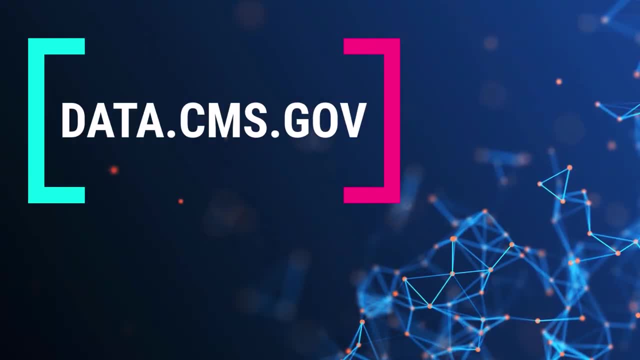 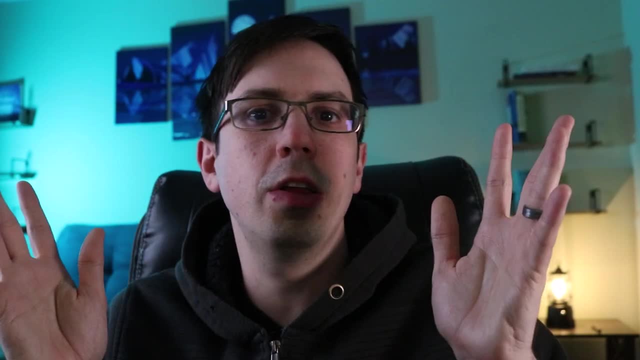 this data set, so check out that video if you haven't already. Next, we have datacmsgov. CMS is the Centers for Medicare and Medicaid Services, and they have tons of free data on their website. One of my favorites is the Hospital Compare data. Hospital Compare is a way of 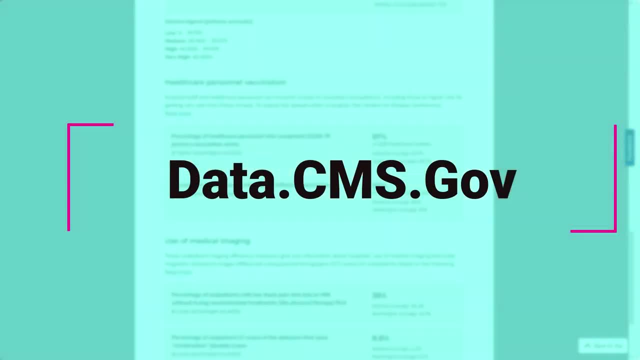 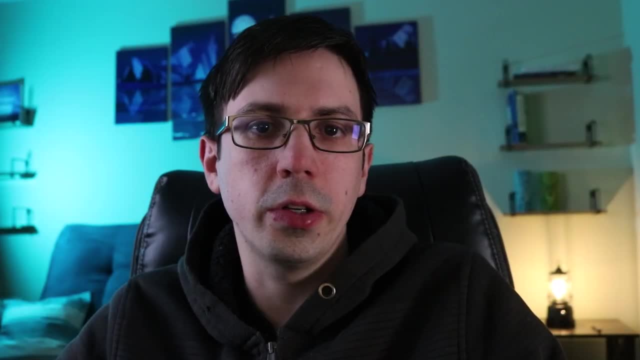 comparing one hospital to another to see what things they're really good at and what things they have opportunities to improve on- Things like patient safety and quality of care. They have an overall star rating for each hospital, which looks at things like how many patients got. 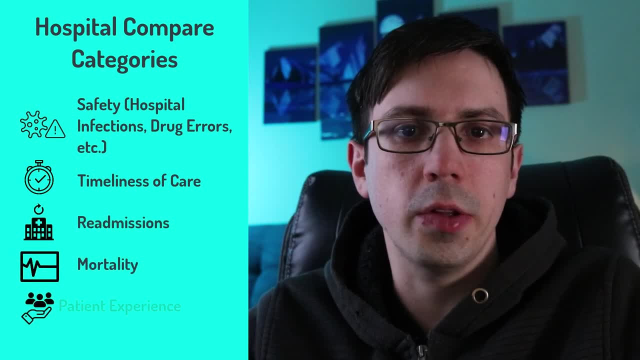 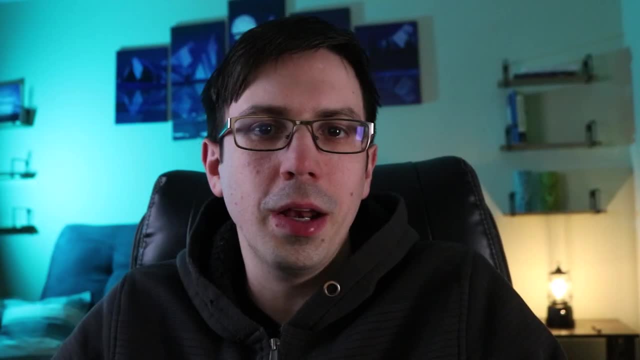 infections while they were in the hospital, or how long did patients have to wait before they got treated in the emergency department? Now, the downside to this data is that they might use a lot of jargon that you might not be familiar with at first, Things like SIR or PSI-90 or fee-for-service. 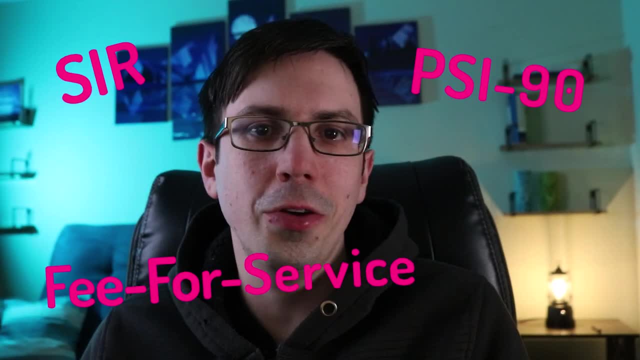 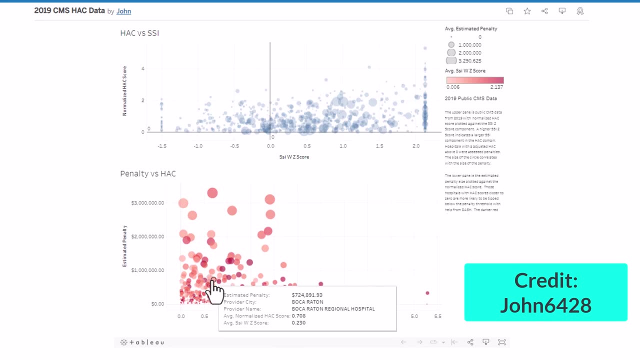 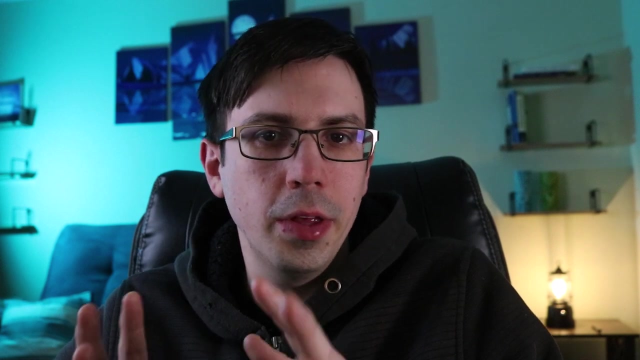 I'll be releasing more videos in the future about this. You might have to do some research ahead of time to really understand what these things are getting at and how to best visualize that data in your portfolio. If you're looking for something a little bit more user-friendly, check out the CMS patient survey rating This. 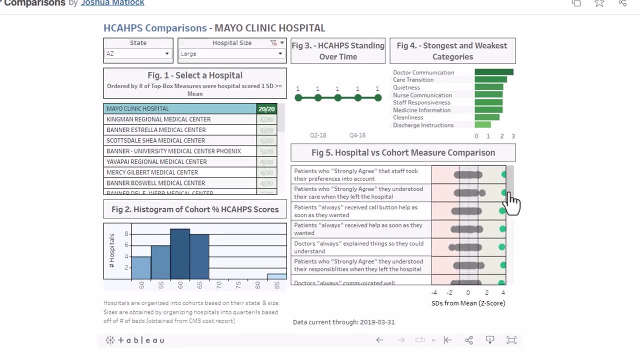 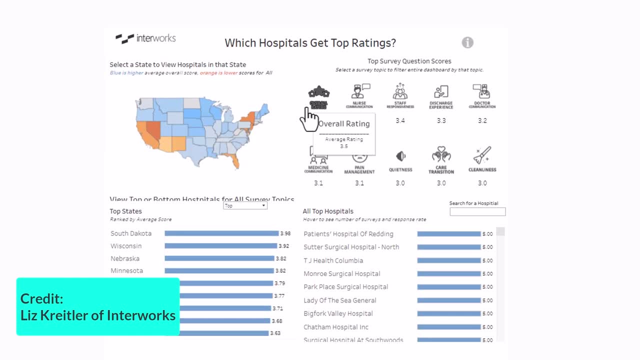 measures, things like what percent of patients said that the hospital was always quiet at night, or what percentage of the patients said that the doctors always treated them with respect. I'm going to have all these links in the description down below, so do check that out. But if you want to check all that out, I'm going to put a link in the description down below. But if you want to check all that out, I'm going to put a link in the description down below. But if you want to check all that out, I'm going to put a link in the description down below. 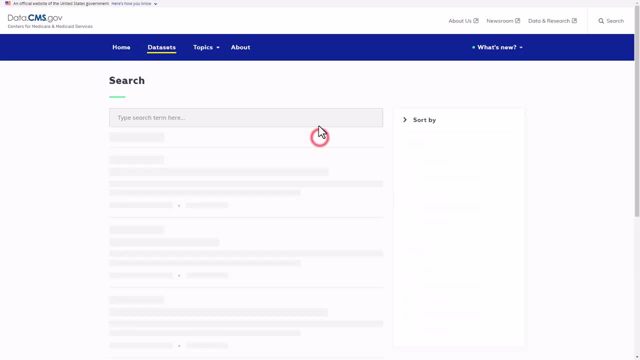 If you want to check all that out, I'm going to put a link in the description down below. You can go to this URL, scroll down to hospitals and then you can look up data sets like hospital readmissions reductions program, hospital acquired conditions and more. 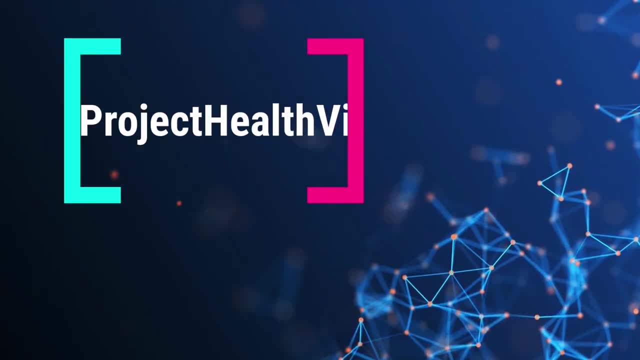 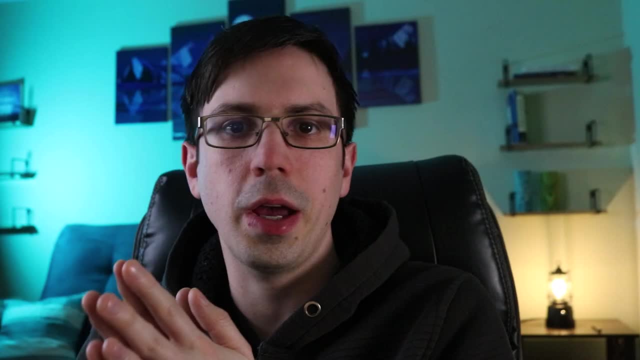 Now I'm going to talk about one of my all-time favorite sources of data, and that's hashtag project health viz. When you're done watching this video, I fully encourage you to go straight to Tableau Public and type in hashtag project health viz into the search bar. You're going to be overwhelmed. 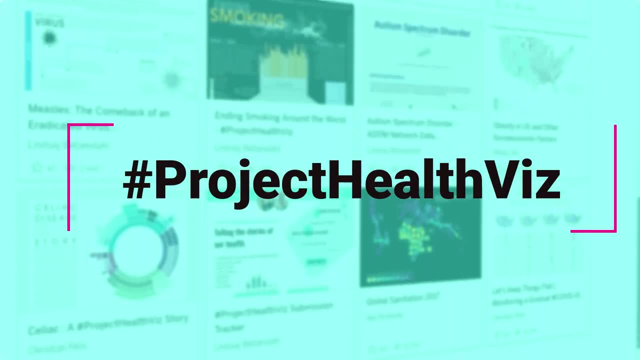 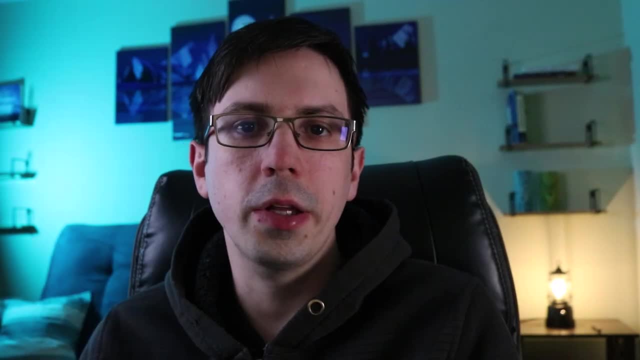 by how much cool stuff there is on there. You're going to be overwhelmed by how much cool stuff there is on there, of the coolest sources of data I think you're going to find- and it's not just one data set, it's a collection of data sets. Project HealthViz was developed by Lindsey Betzendahl, who is 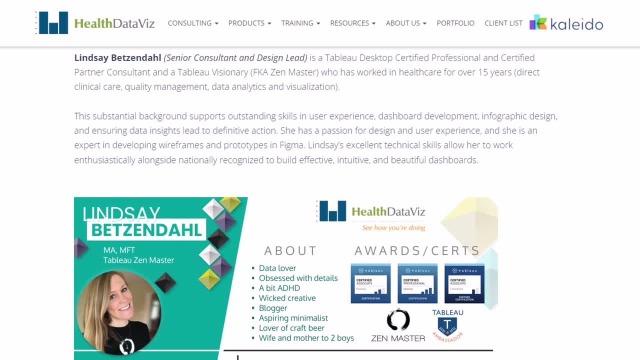 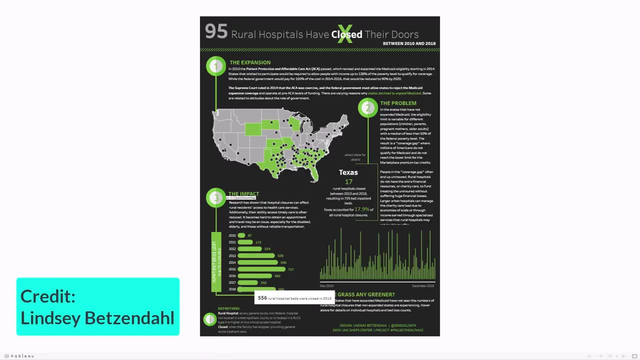 working in the healthcare field and realized that there's a real lack of healthcare data being used in the Tableau community for dashboard development. so she decided to do something about that. Here's how it works: Almost every month, Lindsey is going to publish a data set. That data set. 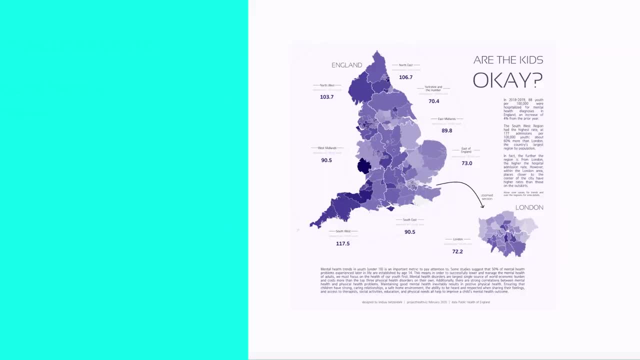 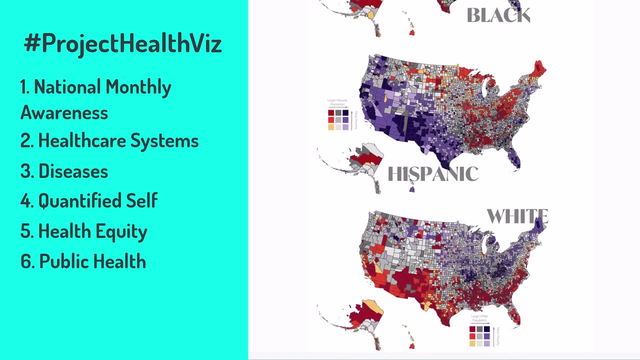 matches one of the following six themes. You have National Monthly Awareness, Healthcare Systems, Diseases, Quantified Self, Health, Equity and Public Health. Quantified Self, by the way, is where people provide their own data. For example, Lindsey made her own sleep data. 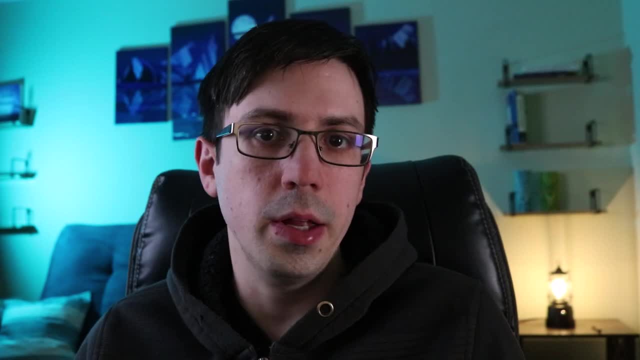 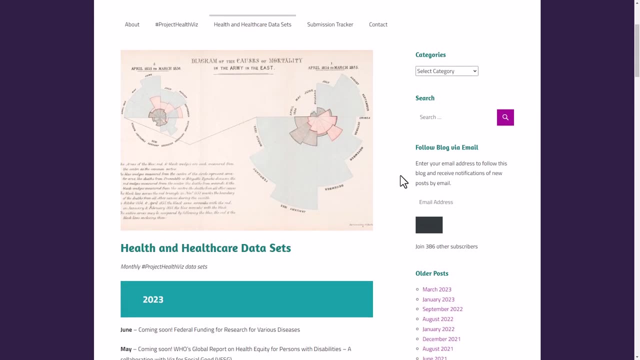 available to the public for analysis and visualization. To get to these data sets, go to her website at vizzendatacom. Click on Health and Healthcare Data Sets and there you will find all of the data sets you need to know about health and healthcare data. 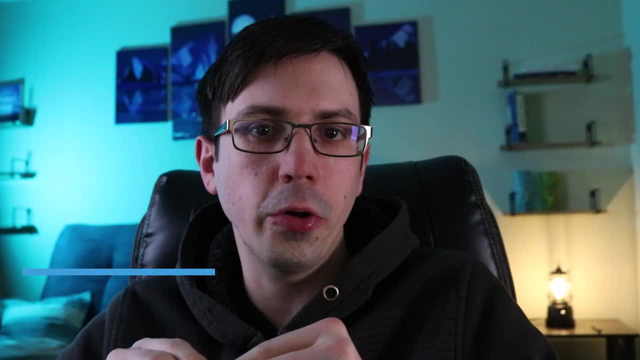 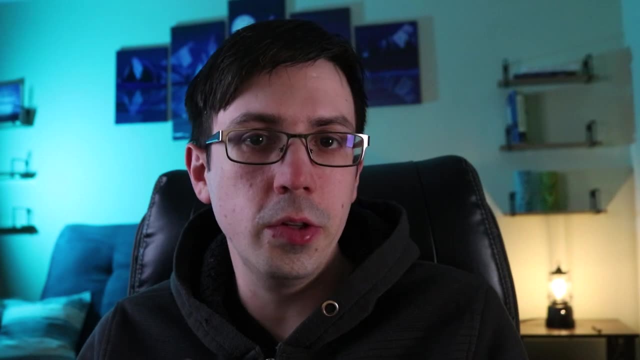 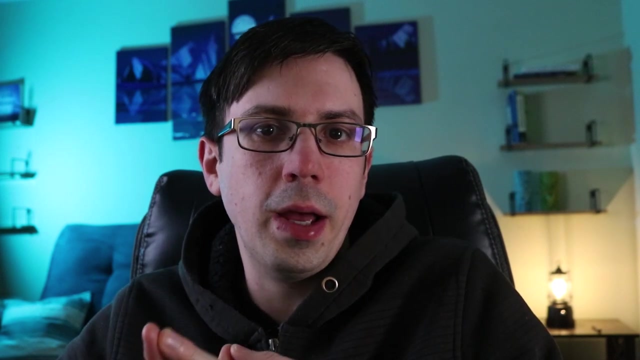 You can also follow her on LinkedIn or Twitter to see all of the new data she's publishing each month. Now, if you're building a portfolio using data from Project HealthViz, I want you to pick one out that corresponds to equity. What is equity, you might ask? Well, equity is ensuring. 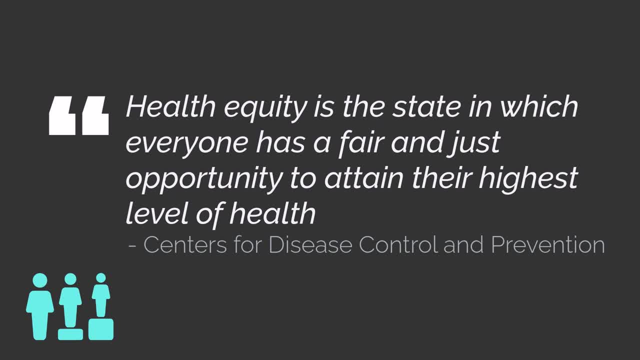 that each person, regardless of their background, can reach their full health potential. For example, as of this recording, there is a brand new data set that's been published called the Loan-Based Data Set. This is a data set that's been published called the Loan-Based Data Set. 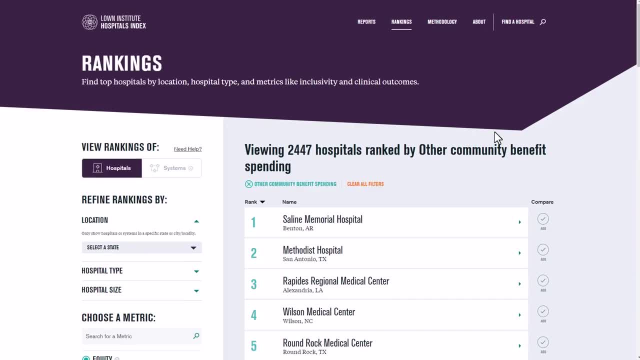 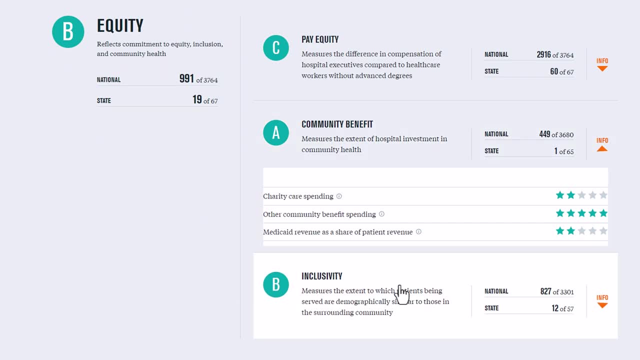 This is a data set that's been published called the Loan-Hospital Index for Equity 2022. This looks at how fairly hospitals pay their employees, how much charitable care the hospital provides to the community and how inclusive that hospital is of patients from diverse backgrounds. 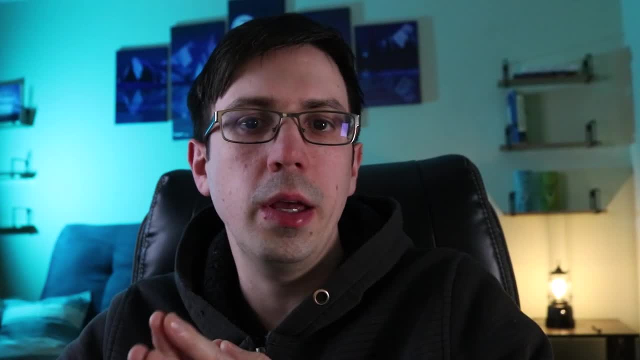 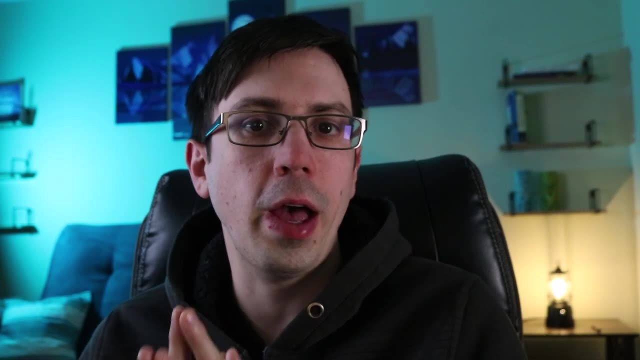 Now you might be asking: why am I focusing on equity? Well, because many healthcare organizations around the country are really starting to recognize how extremely important this subject is. So if you have a portfolio entry about equity and you can speak to it in some way, 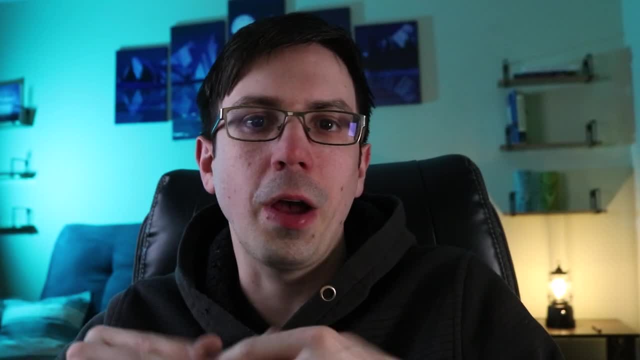 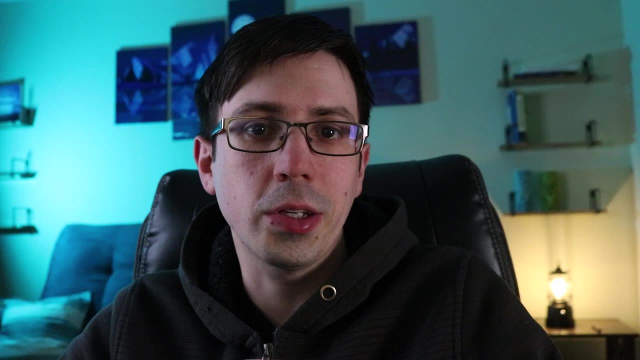 you are going to look awesome during your interview, But in general I like to find a data set that's interesting to me in some way. Then I see what other people have done on Tableau Public. I borrow from some of the best concepts that I see and then I recreate them with my own personal 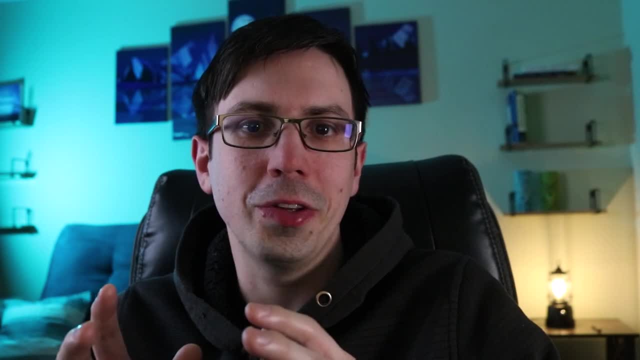 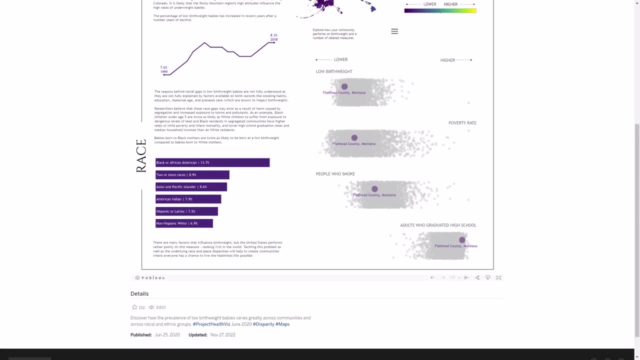 touch, And I think that's one of the quickest ways that you can learn. data visualization Project HealthViz has inspired some of the coolest data visualizations I have ever seen, so I highly recommend that you check that out when you get the chance. Last we have Real World Fake Data by Sons of Higher Ed. 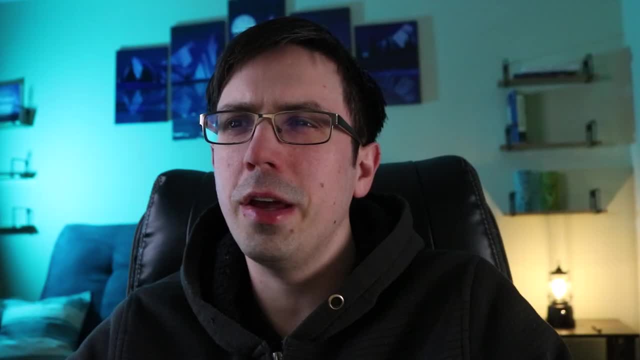 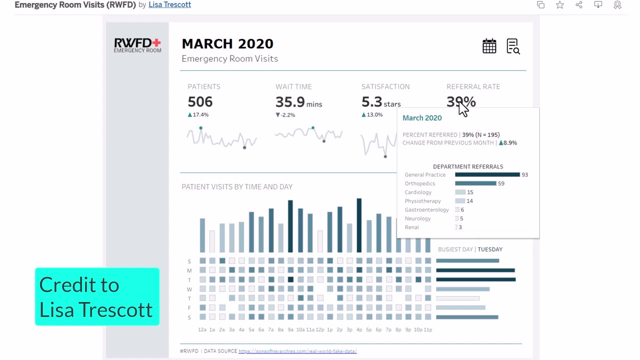 They work with people from many countries across their different agencies and hierarchies. Wait a second. did Josh just say fake data? Yes, I did. If you want to build a public facing dashboard that emulates what a hospital dashboard is really going to look like, you are going to have to use 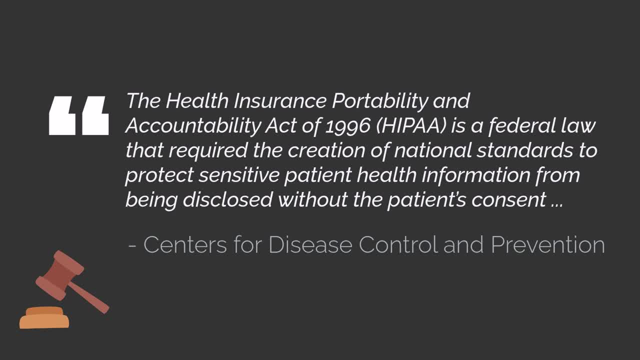 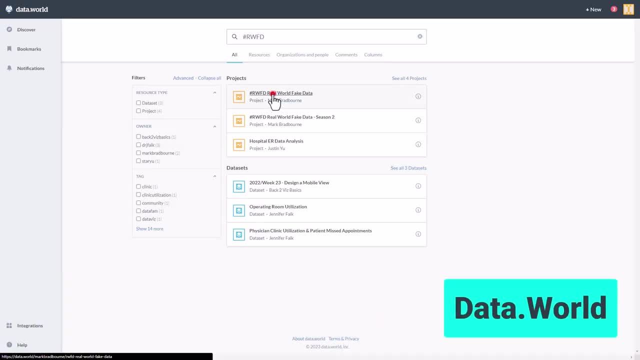 Fake Data because otherwise that data could potentially identify individual patients and that would breach patient confidentiality laws known as HIPAA. Real World Fake Data is a good solution for this. They have a data set labeled Healthcare-Emergency Room. You can access this on. 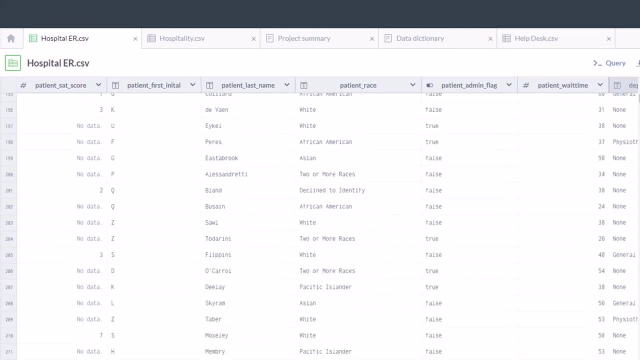 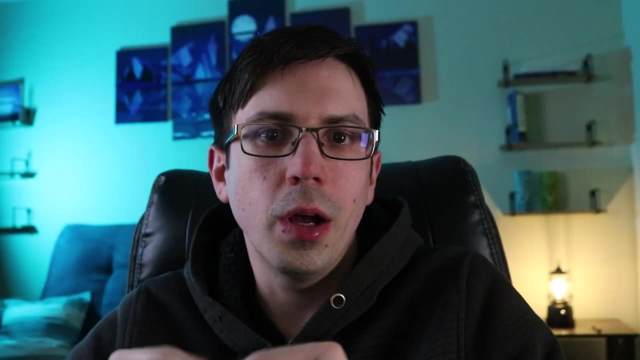 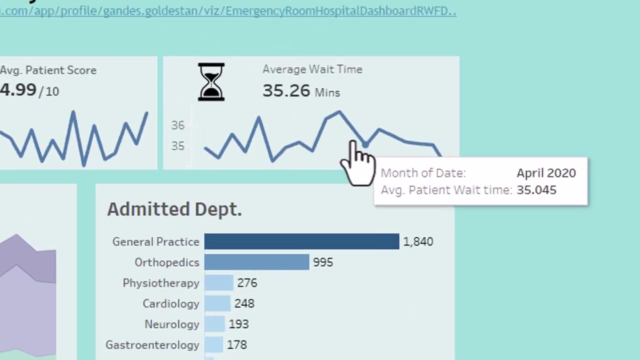 on dataworld. The data has things like patient age name, satisfaction score with the hospital, how long they waited in the emergency room to get treated, among other things. Now, one limitation to this data set is that it's not very real looking In reality. your data in the emergency room is: 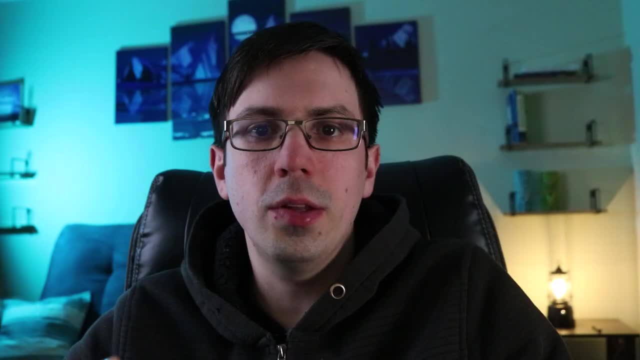 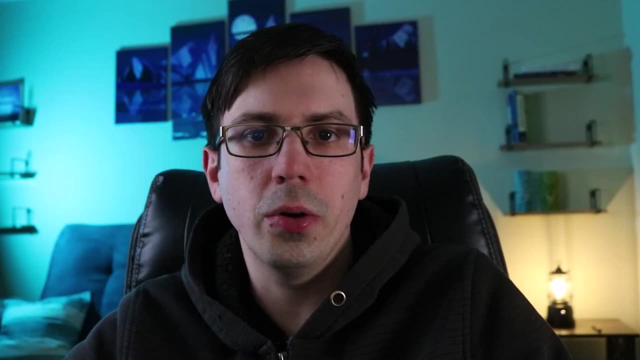 going to look way more variable than this. Here's one example: In this data set, you'll find that there weren't any patients over the age of 79. In reality, you're going to have some 80 year olds, some 90 year olds and even some 100 year olds. There's other things about this data that are 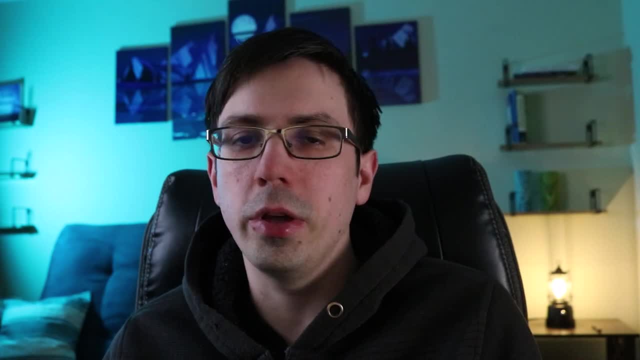 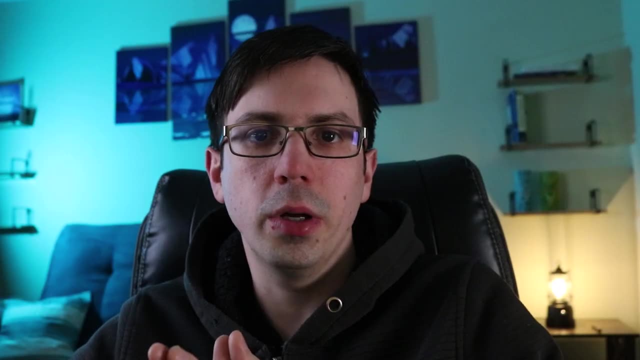 unrealistic, but for the most part it's a pretty good mock-up of what you might expect to see on a hospital dashboard. There are some really awesome looking dashboards that use this data on Tableau Public. that will inspire you to make your own awesome dashboards, Speaking of which?